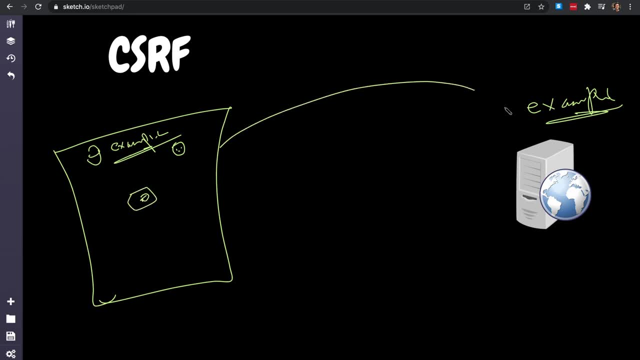 a button that says get- I don't know orders, right, I'm going to make a request and, since the HTTP protocol is stateless, it's going to send all the time. It's going to send the cookie here, right, I'm going to send the cookie here, and that's how the server actually recognized me. 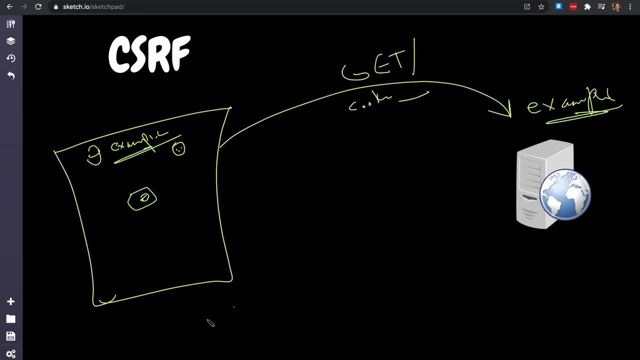 Cross-site request. forgery is the ability of a completely different site- here evilcom right- Having the ability to send a request on your behalf while sending also the cookie right. So somehow this website, which is the evilcom, managed to get your cookie and when it does that you can. 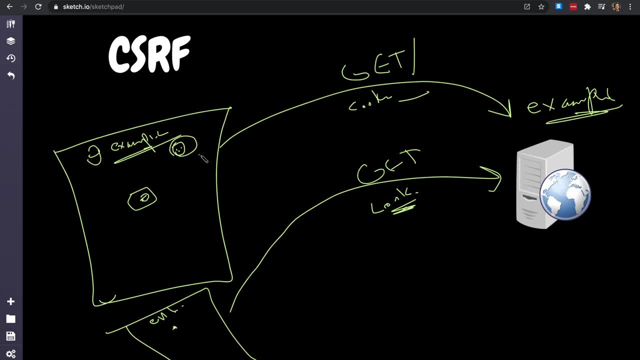 the site can actually make requests on your behalf, right? So this could happen even by even just clicking a link going to that web page and that website when it makes a request to examplecom, if the browser was dumb enough to send that cookie- and we know cases where this is actually- 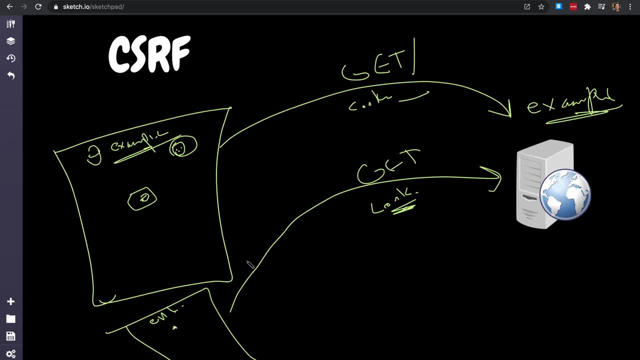 possible, right? For example, if the same site cookie is none, then we always going to send that cookie, right? We talked about same site. go check that out. We talked about same site. go check that video out right here. but yeah, cross-site request forgery can happen as a result. This is one. 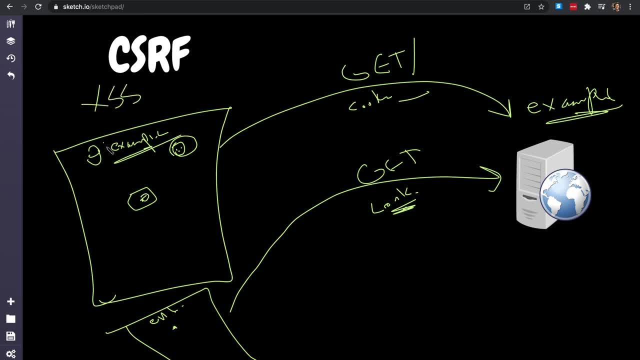 example. Another example is XSS: right, Cross-site scripting. Is that how you spell? Yes, Cross-site scripting. right, So I am. this is even more dangerous, right? So cross-site scripting can allow the user to inject code into your application, right, And when you? when? 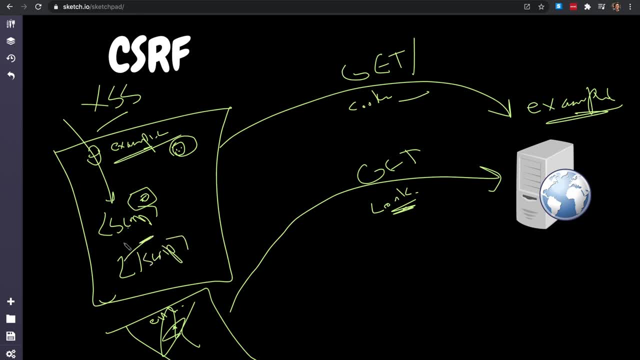 i, as a bad actor, i inject code into the application. i can make requests on your behalf in the application, and even the same site property for the cookie will not protect you. this cross-site request scripting is the worst right. that's why we have to sanitize input. you have to do all that. 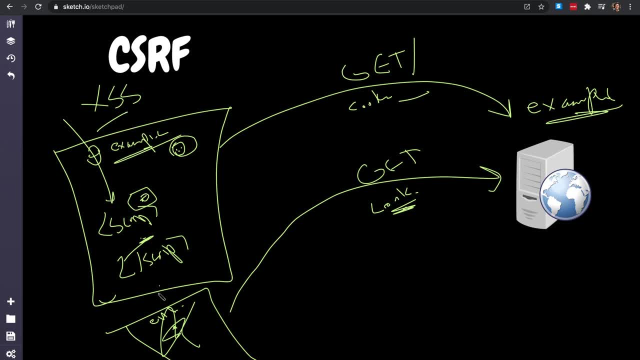 stuff here, right? so yeah, cross-site scripting or that can lead cross-site request forgery. so the attacker is forging a request. so technically you didn't make that request. right, this request is evil. but someone else made that request on you on your behalf. they forged the request and it happened. 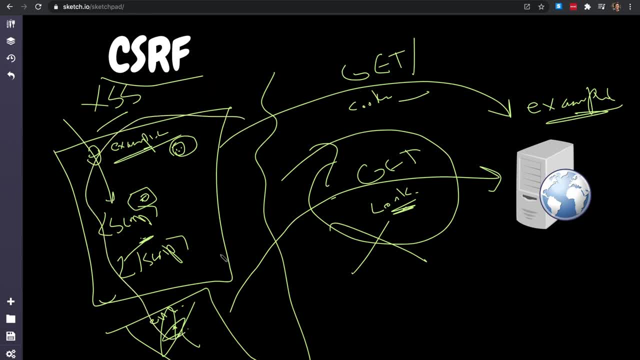 completely at the client side. that's how i remember. cross-site request forgery, so it's a cross-site. well, it can happen in the same site as well if you injected some xss and you send some results here and posted it on the client side. so it's a cross-site request forgery. so it's a cross-site request forgery. 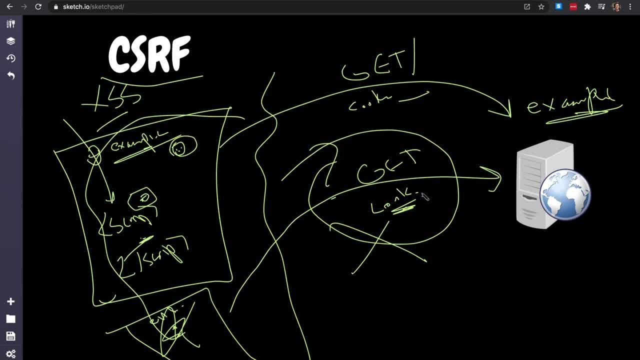 the output somewhere else. you might say: what? what's wrong with making a get request to get an order? well, this site can get the request and display the orders in their website and then save it to disk right. and then, uh, not really save to this because it's your disk right, but, yes, it saved. 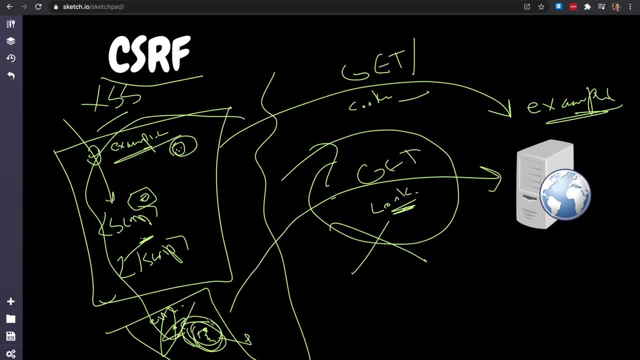 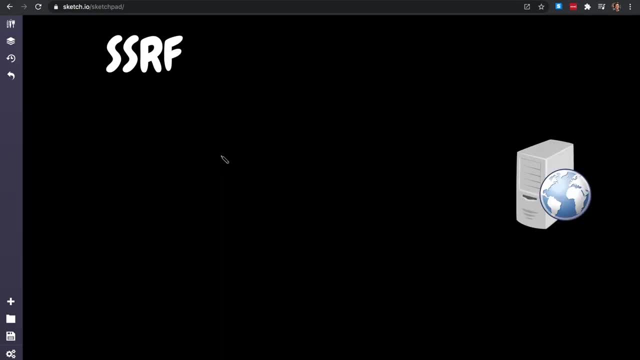 it can have the information locally and then upload it later to their evilcom website. all right guys. so that was the cross-site request forgery. real quick, all right guys. uh, server site request forgery is is one of those names that i believe they are given name for the sake. 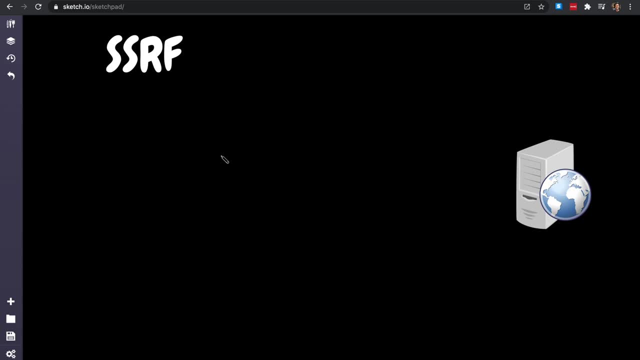 of just having a name. to be honest, i i don't think they deserve a name. but sure, since we name everything on the web, let's, let's name this attack too. so server site request forgery is the ability of. the forgery is happening on the server side, so let's, let's explain what that means. so let's. 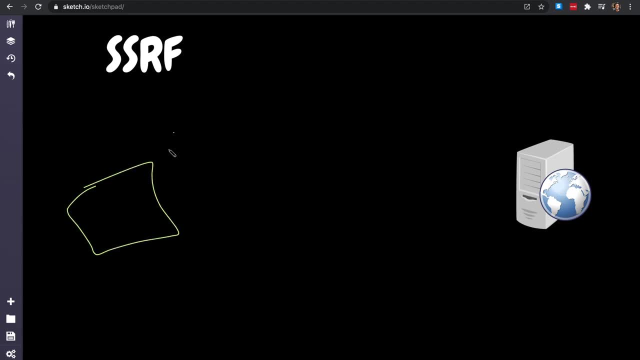 assume you are a client here, not necessarily. obviously, web server or browser is just a client- and uh, we're making a request and the api here- that api that you make a request to actually the server is- is designed to make another api to other servers. right, let's say this is another server, all right, so this is the api. let's see this is. 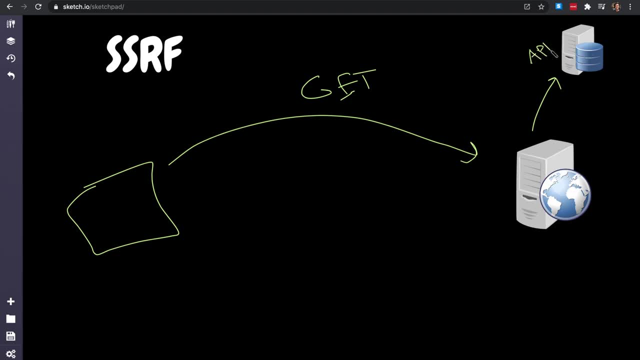 not a database, right? let's say, this is another api server that happens to i don't know check the prices or something, right? so that to make this git request successful, the server take that git request and makes another call to another api. this is how microservices. 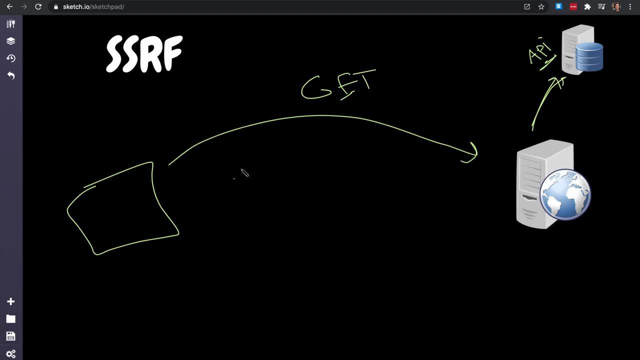 does all the job most of the time- some implementation. if if you have implemented this in a way such that you actually specify the api, the back-end api, as part of your body or part of the url, even get request or post request, let's say, let's say this is http. 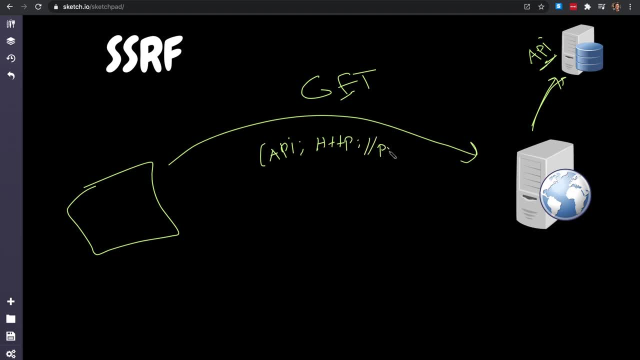 pricecom- right, this is the api, whatever apipricecom, and this is the, the server of the price dot com api. right, that's the server. so what do you do is like, hey, i'm gonna, i want all the products right and here's the api for the price, right? i have no idea. why would you do something like that? 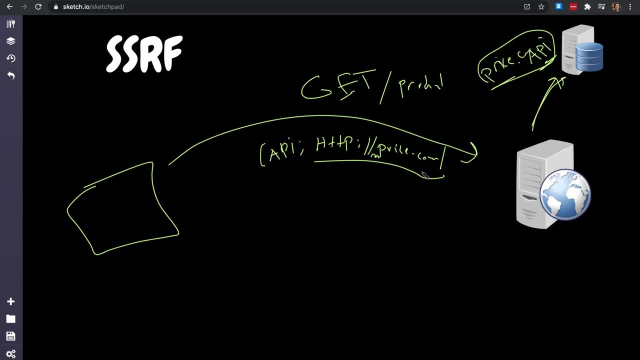 that's bad practice in general, but some apis does that right. they actually make for flexibility reason you you can specify your own api if you want, to what api endpoint you want to use. if you want to do that, never actually specify the url. that's the problem and we're going to explain why. 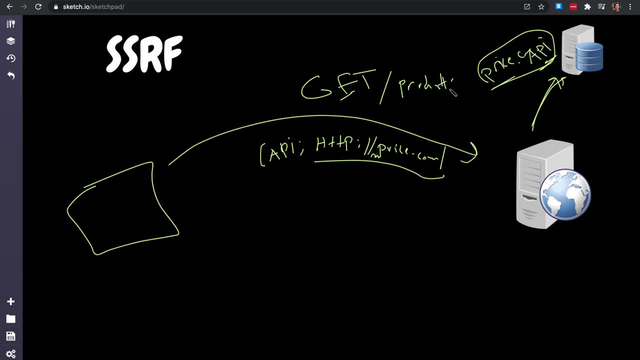 in a second. so what? what happened here? i'm making a list, all the products- and the server will say: okay, i have the products right here because i am local database, but to get the prices of the product i need to call in the priceapi product, get that result, cache that result and then response with. 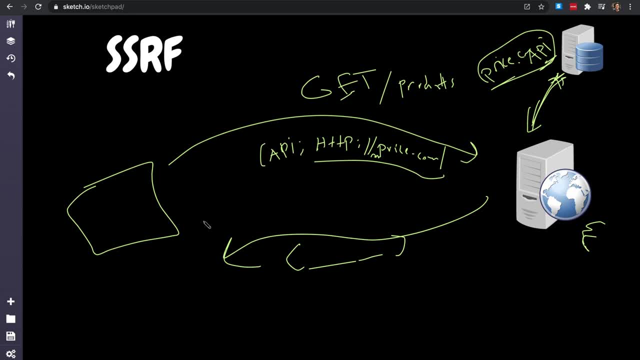 everything to the client. so what's wrong with this, hussein? so here's, here's the problem. right, since you gave me a big hole, right here, i can specify anything right here. right, i can specify http. i want you to go, i want you to make a call to localhost slash admin. right, or one, two, seven, zero, zero slash admin. and what the heck is. 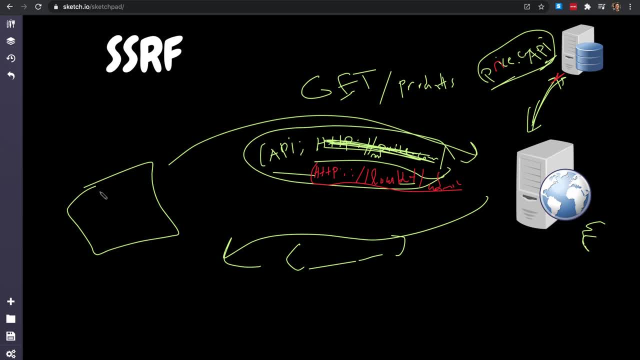 localhost. if you make a request localhost right here, it's going to fail because you you don't have anything running right. however, if you don't have a localhost, you don't have anything running right. so i'm going to go ahead and do that. i'm going to show you, you know, if you don't have a localhost. 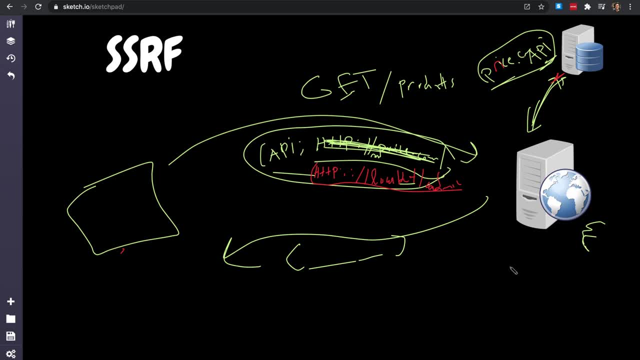 you can simply right click what you tell it and type in like uhm, and here's $none. but you don't even have to type $none right to get his where all data. and then I need to make sure i have got all密 right and here it is, and I you know it's working and so i will go ahead and show you right now. 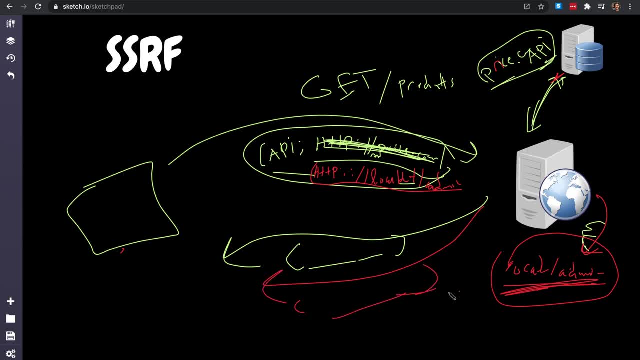 so what's going to happen now? let's see what's going. sort of behind, you goes over here. let's take a look at our solutions. first timeuber, now that we've it's going to return all the content, right, because you don't have to log in, because you're admin. 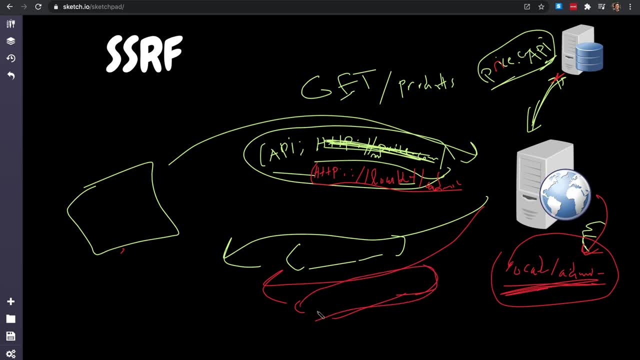 you're literally in the admin space, right? that's one way of doing so. so what happened here? the server is doing the forgery, right? this? it's a server side forgery- request forgery. so we're making a legit request as far as we are concerned, right? however, the server is making that forgery. 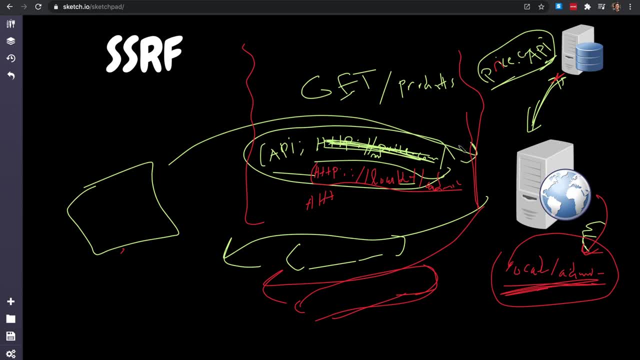 right, the forgery happening in the server side, right it's. it's purely a bug at the server side, right, because we're allowing that. so another thing we can do is i can, for example, allow http slash, slash- what uh? another website or server that only the server have access to, right, i don't know. 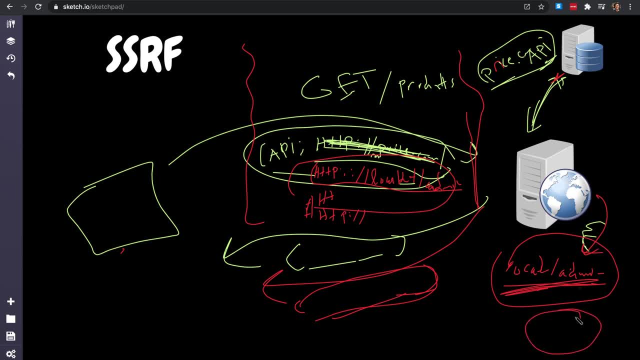 some other services here that is private to this resource. right, you can just make a request and it will send you a request, and it will send you a request and it will send you a request and pull that information. ftp perhaps? right, pull an ftp service and pull some local. 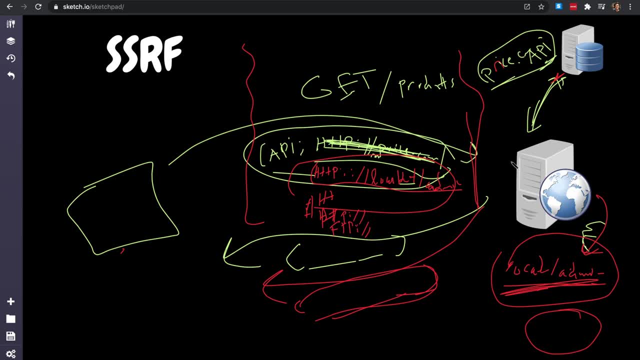 resources if there is an ftp service running around so you can make requests on behalf of the server, and that's extremely dangerous. you can go all the way and if you get- obviously you gotta get the admin result or get the ftp result- you can go all the way also and make a ddos attacks. 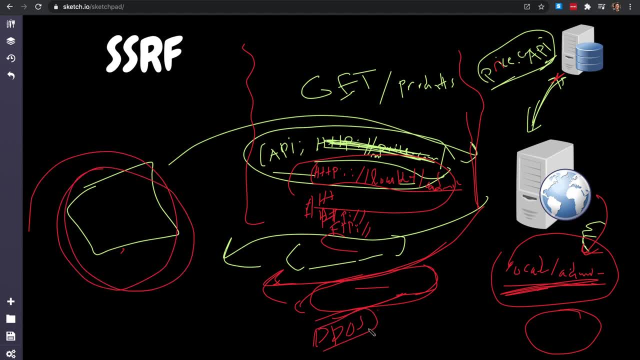 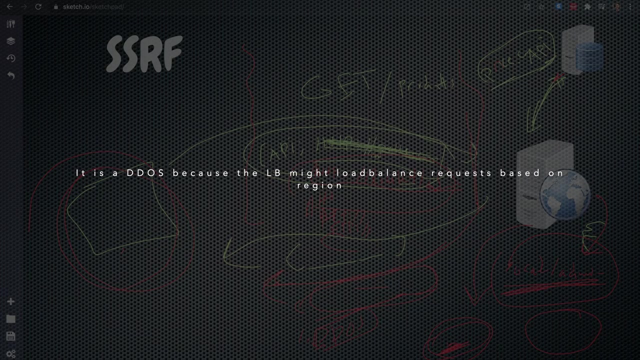 if you own many of these requests, you can. you can essentially ddos a poor slop right here a server, that is just completely normal and make a request so that the server makes that request to the sir, to that uh third party service that you want to take down instead of you. so that's another way where server side request forgery. 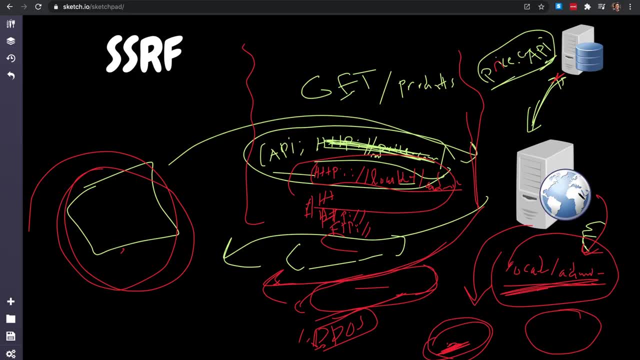 also, uh, can take effect right. so in a short guys summary, all right. so quick summary, guys. cross-site request forgery: the forgery happening at the client side. you are as, as an, as a bad user you are making, you are hijacking an authenticated user, an already. 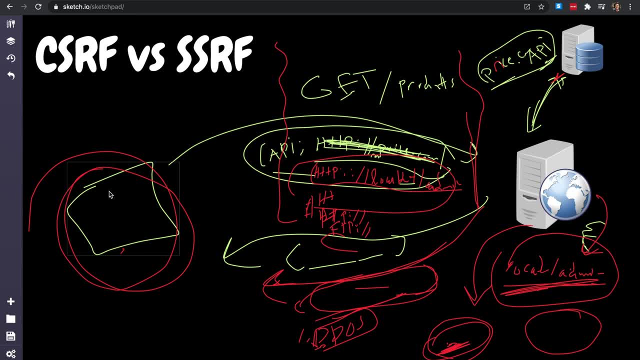 authenticated user request and making a request on on their behalf. so you're making at the cross side, at a client side, right the server side. you are just a normal, you are the bad guy and you are connecting to the server as the bad guy. you are just a normal, you are the bad guy and you are. 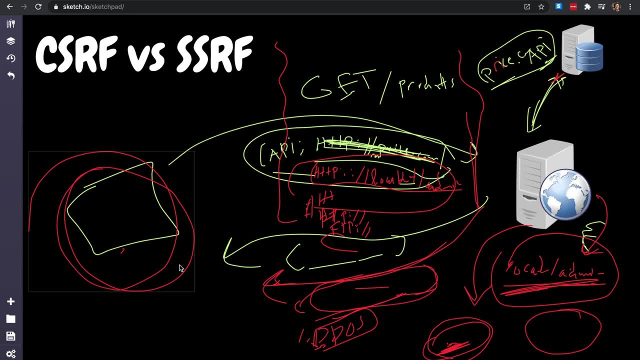 right, and you are making a request and forging the request at the server side, right? so you don't really. and the server side request forgery is more dangerous because you don't really care about cookies or anything. you don't need anyone authenticated. you can do it yourself as a bad user. 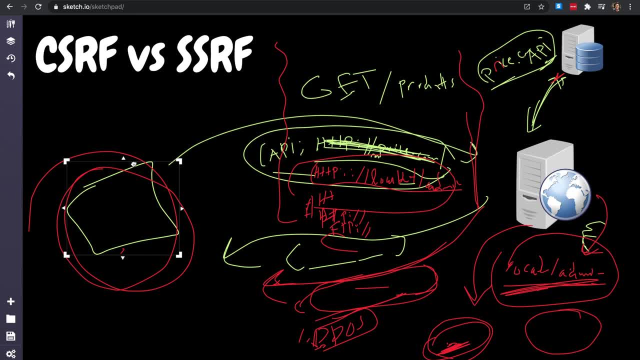 as a bad hacker. right, you can just hit the server immediately and just do the bad stuff immediately with the cross-site request forgery. no, you're hijacking an existing user and login. right, you're sending a user, someone and it says, hey user, go ahead and uh, click on this link in emails, right? 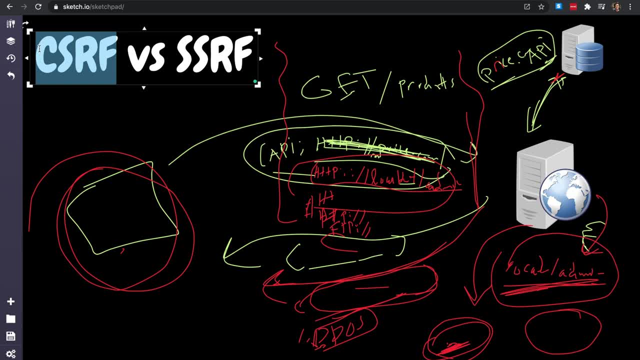 for example, and: and this way they you can do a cross-site request forgery. well, the server side is like: so back in, engineers, guys, you have to watch out for this. front-end engineers, you have to watch this for this, right? this is for back-end engineers, this is for front-end engineers, right? 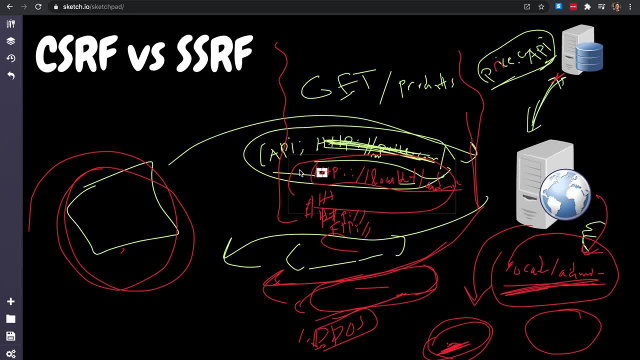 so back-end engineers make good apis never, never let the client specify a url. always specify, i don't know, some sort of a lookup right. it says, okay, the pro price api, and then look it up at the back end. if it's not supported, return an error. never allow your apis to expose uh. 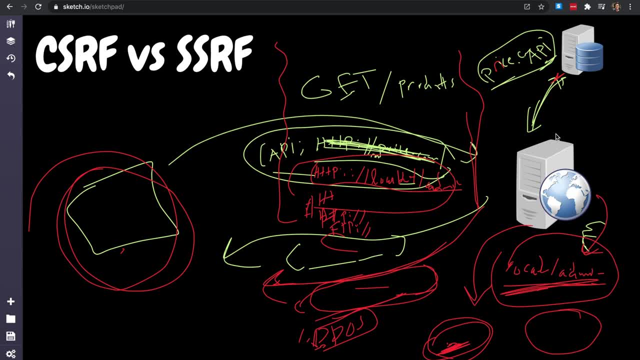 essentially just plain urls, all of uh, just like that planes there. so yeah, so server side versus client side. guys, hope you enjoyed this video. very quick. i'm gonna see you on the next one. you guys stay awesome, goodbye. check out the other content in this channel. i have a. 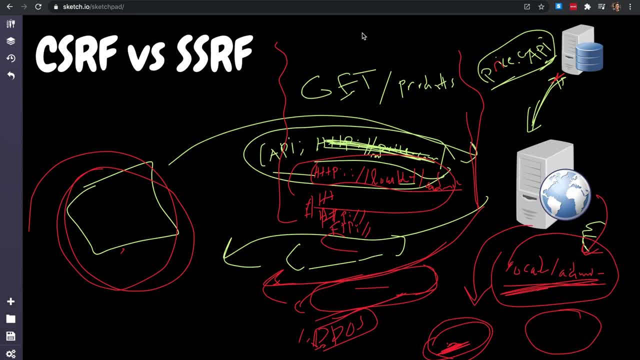 treat all the love and subscription guys. goodbye stay awesome.